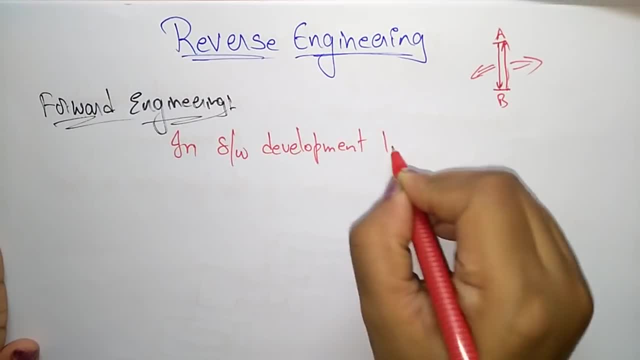 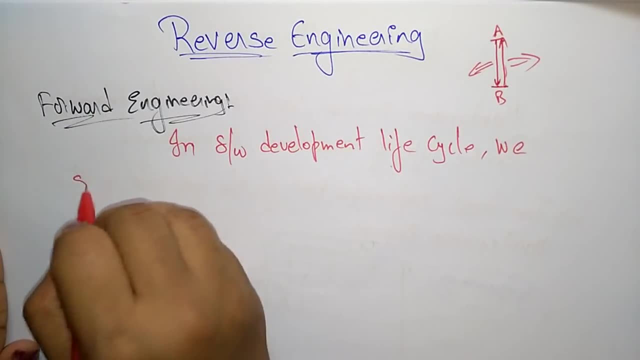 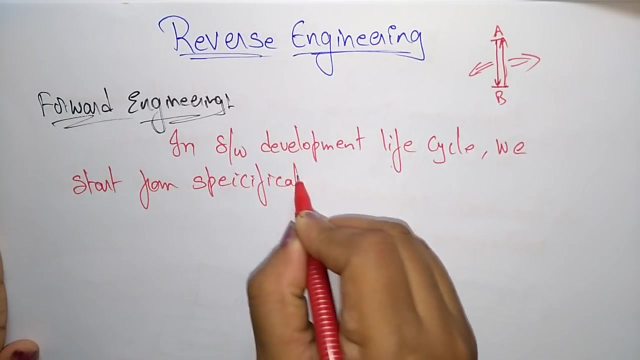 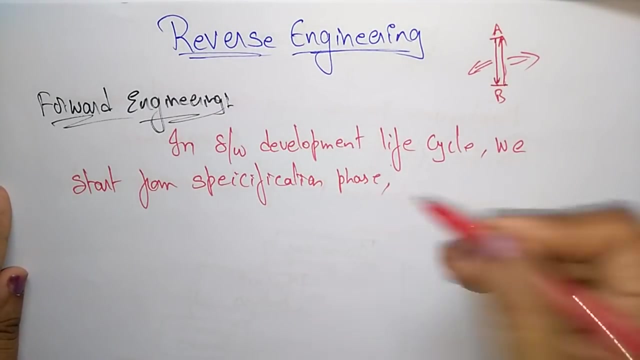 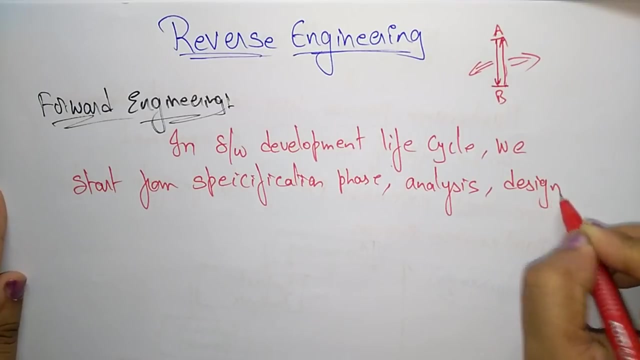 So in the in the field of software development life cycle, in software development life cycle, we start from. We start from Specification phase. Okay, we start from starts from specification phase and go through analysis phase. So after that, Analysis, Design And implementation. So this is a normal procedure- means: whatever you have taken the project, what type, 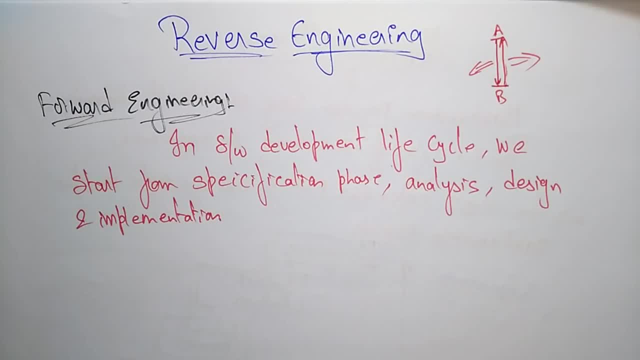 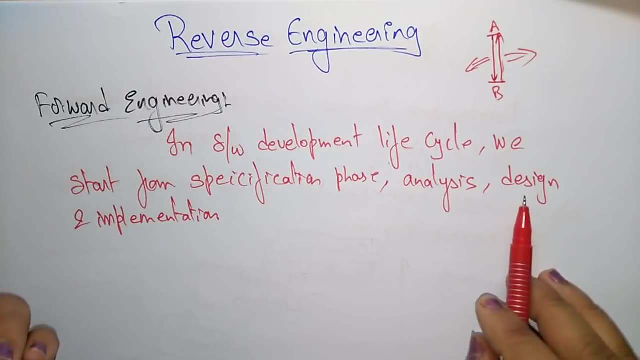 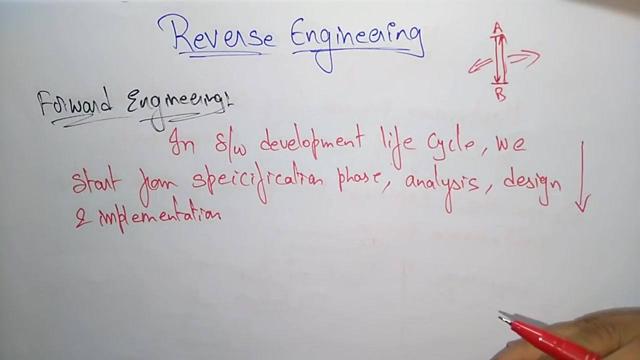 of model you have taken. you will follow these specifications means from start, from the specification Phase, means that is a requirement gathering. Next you have to analyze the document requirements and after that you try to design the project and after that you have to implementation and testing. this journey of software development life cycle you call it as a forward engineering. we are following one. the specification means one method, so everything will be: starts from gathering the requirements and ending with testing. then what about the reverse engineering? 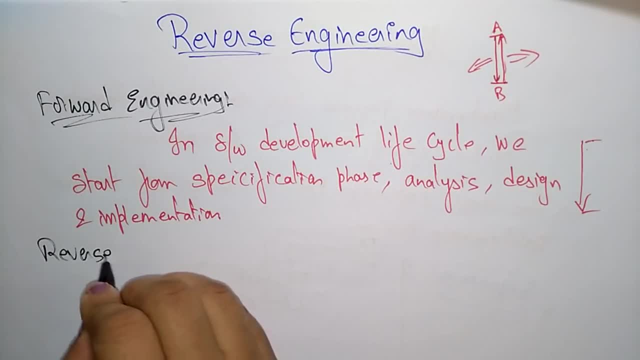 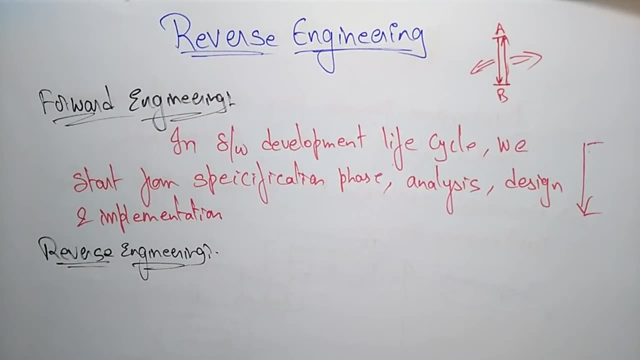 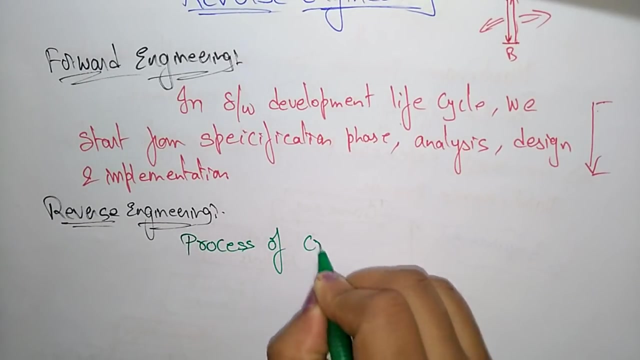 So everything will be starts from gathering the requirements and ending with testing. then what about the reverse engineering, Revers, Eng. Revers engineering means process of creating. Let me write that process of Creating Of design document, Process of creating the design document. 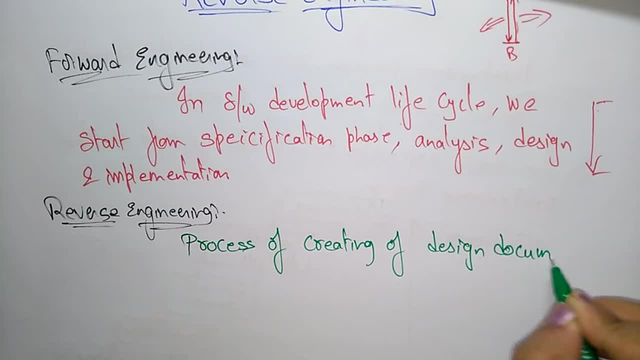 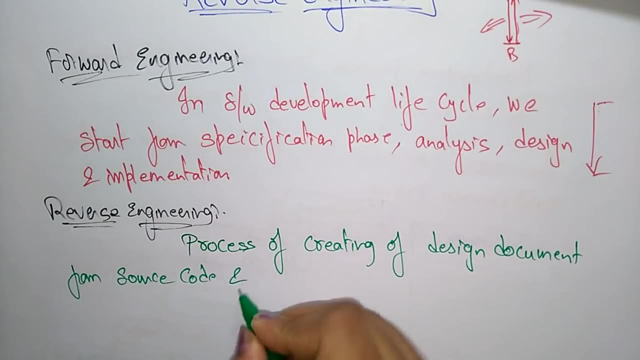 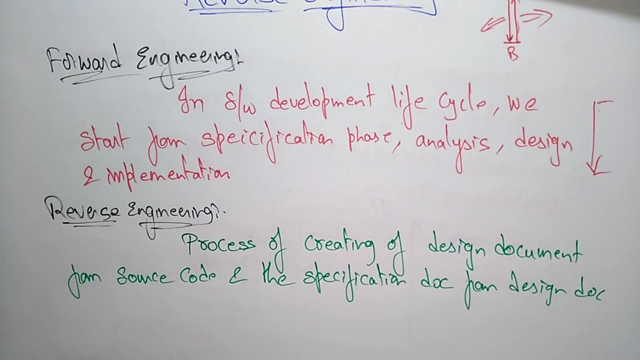 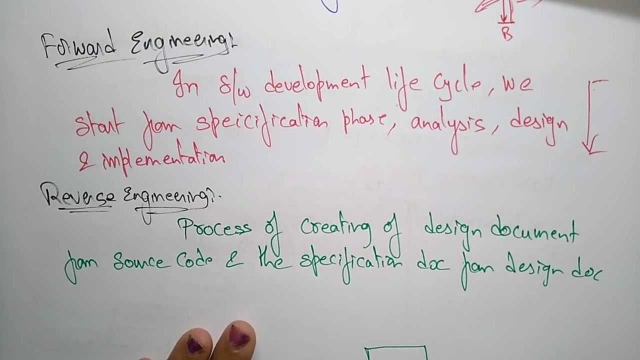 From source code, From Source Code, The one of four Design Drawing Colony and the specification document. and the specification document from design document, from design document. so this process- you call it as reverse engineering- what i am saying here, the process of creating the design document- how i am creating the design document? by taking from 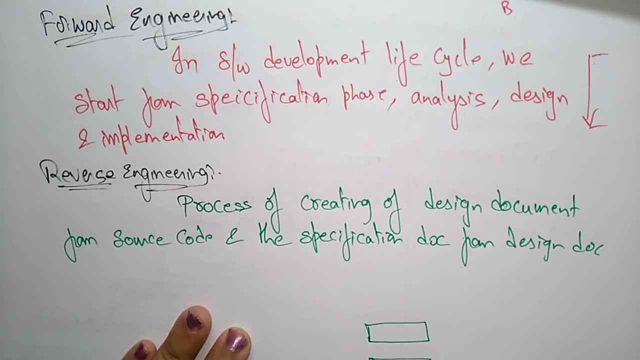 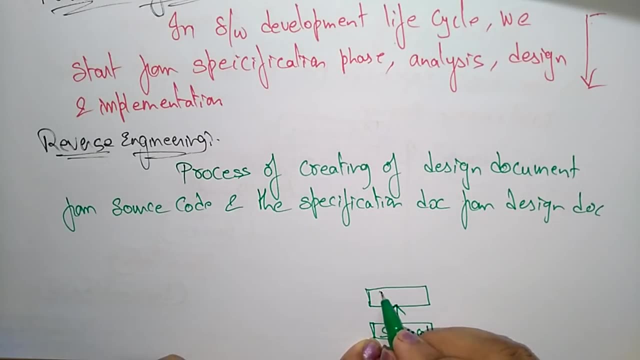 the source code. so here, the source code is there from this source code. okay, a source code will be there from this source code. i am trying to design the document from taking the help of source code, by seeing the code only. i try to design the document and the specification document from. 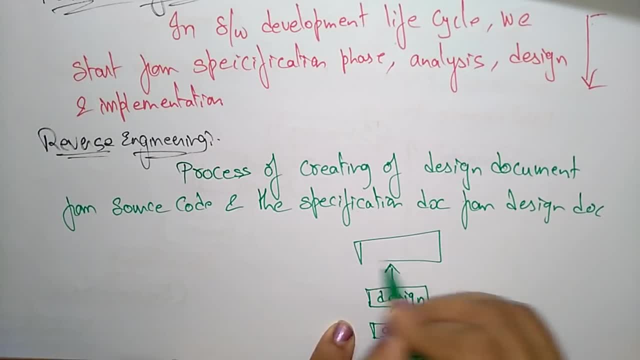 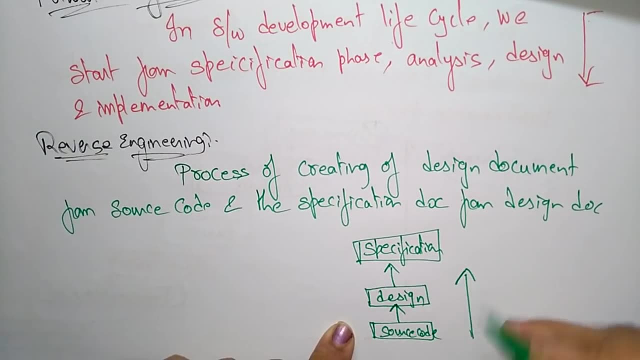 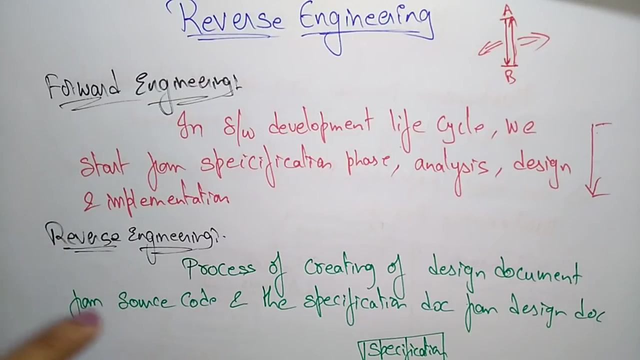 design code, from design code i try to create the specification document. so here it is, following the reverse condition. so this is a forward condition and here we are following the reverse condition. so this is the main difference between this forward engineering and the reverse engineering. so here starts with the specification and end with implementation, and here we are taking the. 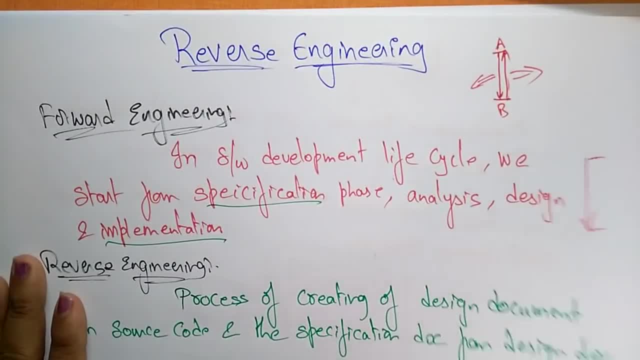 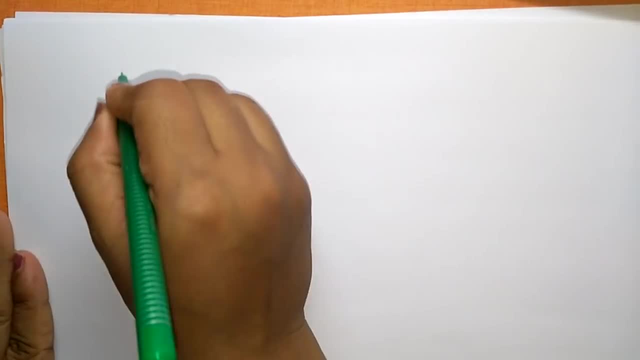 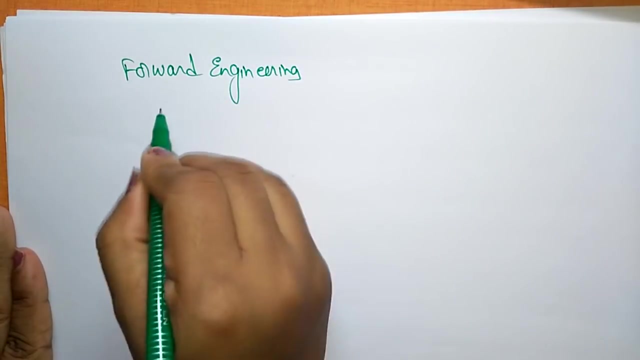 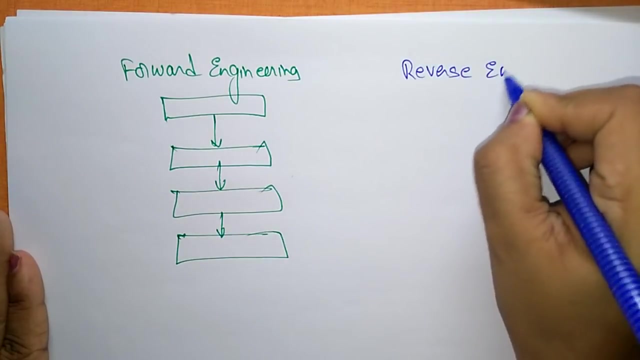 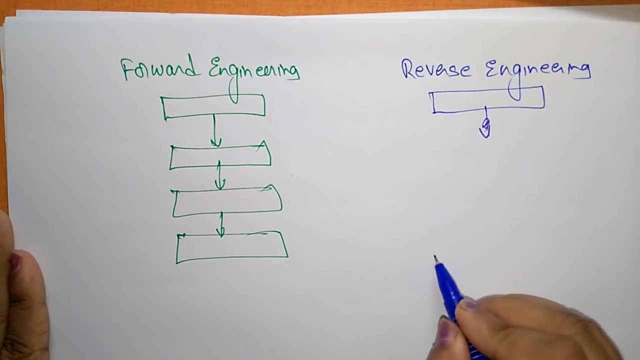 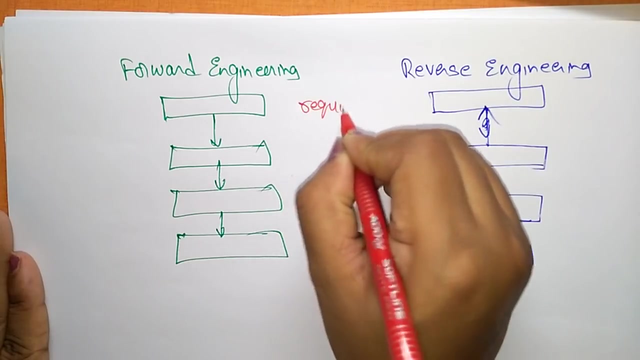 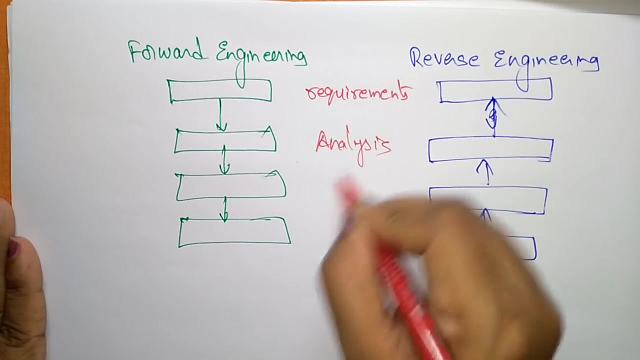 implementation code and try to develop the documentation. so let me write that here i have taken the forward engineering and next here reverse engineering, reverse engineering. so in reverse engineering also you are having four phases. sorry, this direction, okay. so here, first, requirements, requirements analysis phase, design phase and implementation, implementation phase. so in the forward engineering first we are: 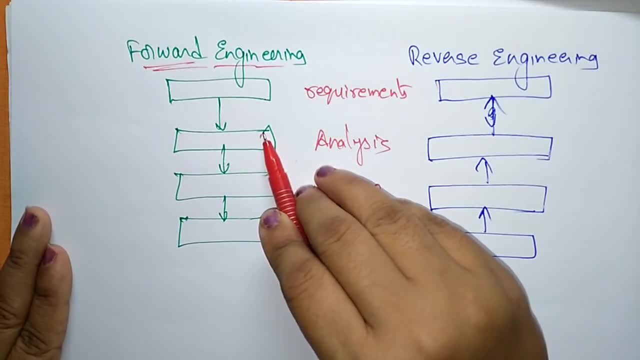 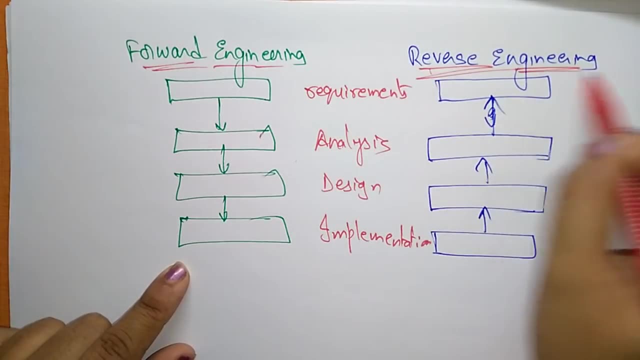 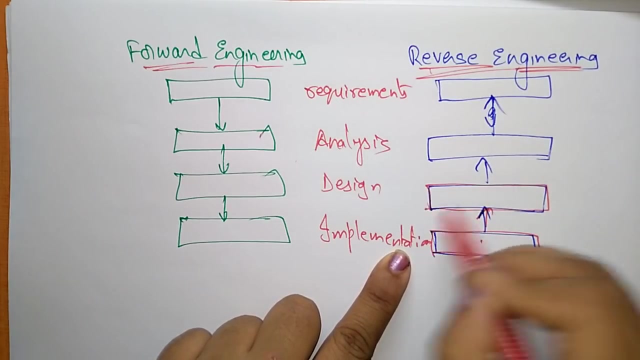 gathering the requirements. after gathering that, analysis will be started. after analyzing, design will be started. after designing, implementation is started. but in case of reverse engineering, first implementation has taken from by seeing the implementation. they are trying to design the product. okay, design after designing, they try to analysis. so what i had, what the design i have taken, what design i created? so 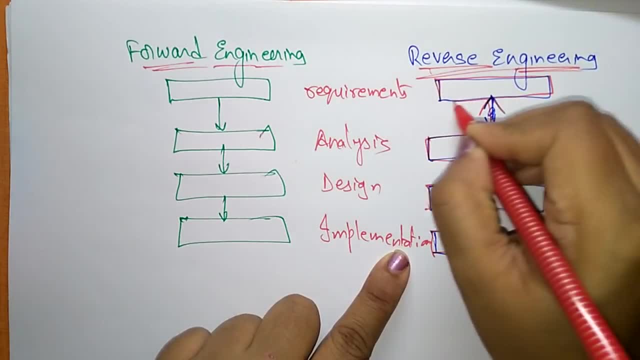 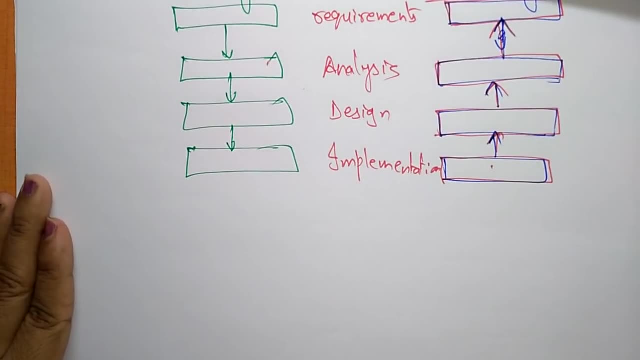 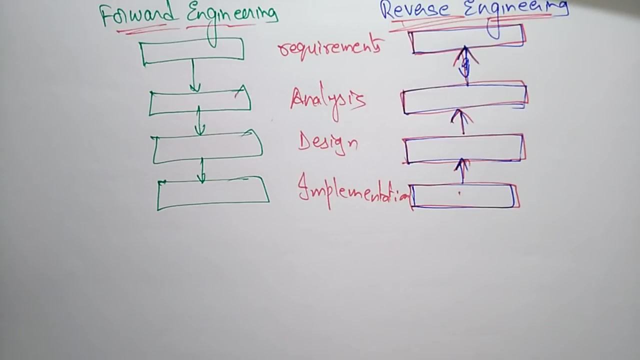 analysis product and give this requirements the specification document to the person. so, man, so this is a reverse engineer. now let us see why we are using this reverse engineering. so in which fails is reverse engineer, so in which feels is reverse engineering. will be useful everything every where we fall, following the forward engineering only. 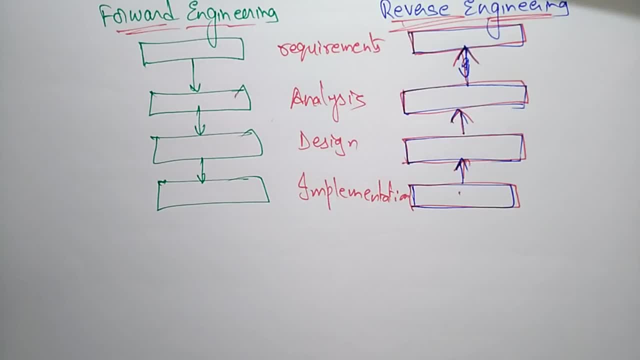 so, whatever the product that we want to be, double up that you have to follow the forward. ensuring means by taking the requirements, analysis, designing, implementation. so that is a regular process. then why we are going for the reverse engineering, in which cases it will be suitable. now let us see a. 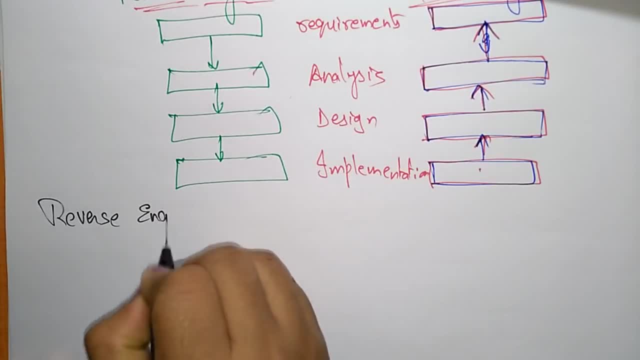 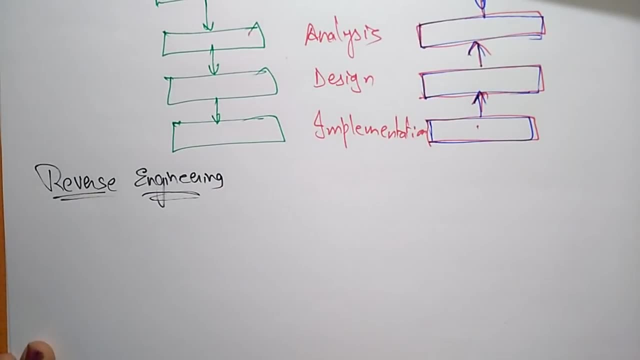 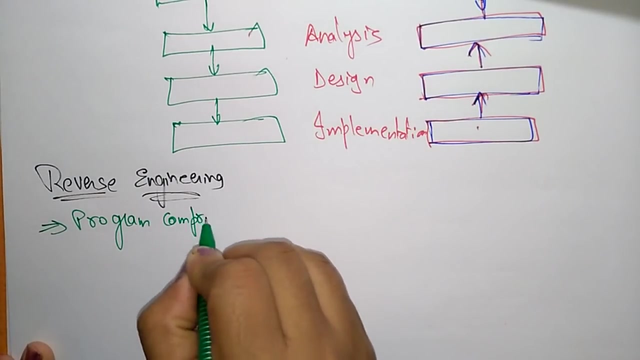 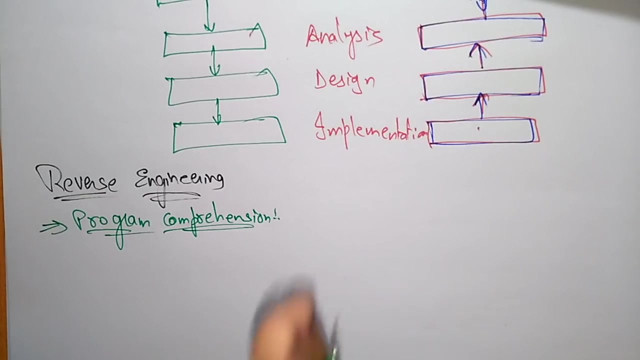 the reverse engineering. so in the reverse engineering, first you are having the program comprehension. let me write about the program comprehension. so what is the use of this program comprehension analysis, existing software with the view to understand its design and specification. so first you have to take the existing software. so from this existing software with the view to 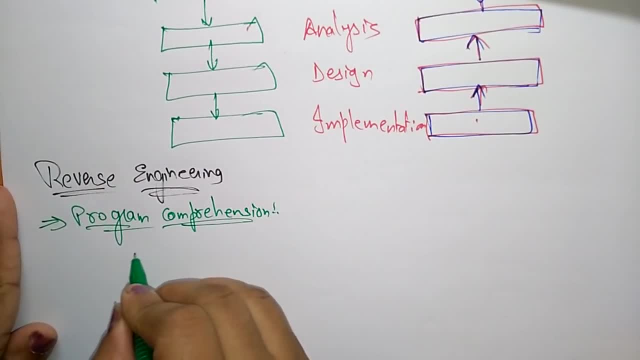 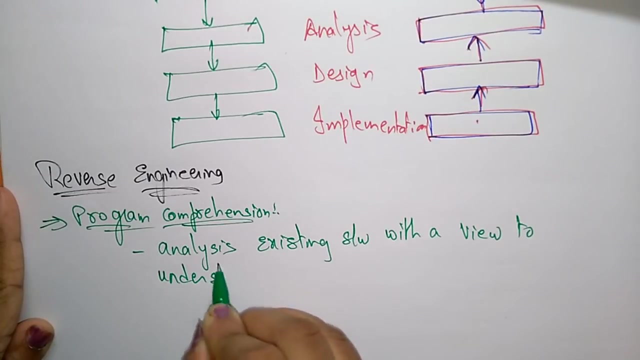 understand its design and specification. just analysis existing software with the view to understand it's design and specification means, uh suppose, if you are seeing any existing system, uh, whatever the existing system you are taking, any app you are taking, you think about so how its design will be. 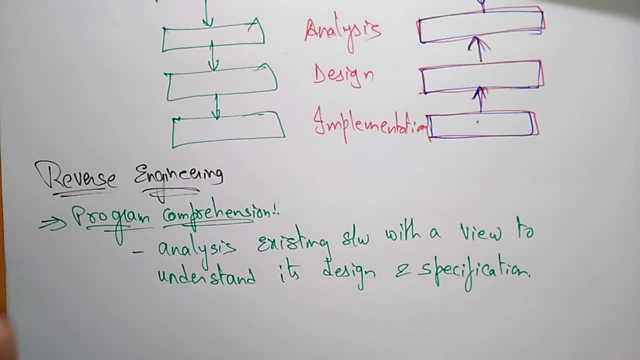 and what are the specification. so, on what specification they are trying to develop, they tried this uh software. so that is a way of reverse engineering. by taking the existing system, we are trying to understand what are the designs for this existing system and what are the specifications for this existing system, how they reached this existing system. so by following the reverse 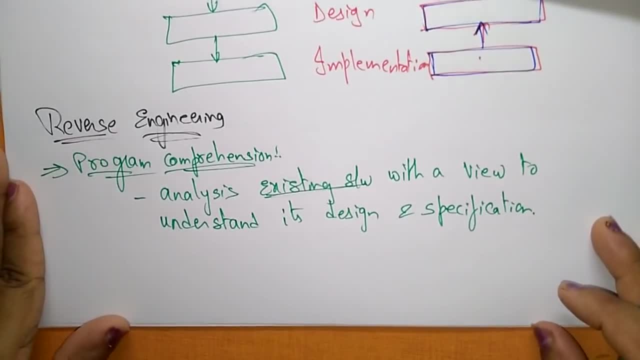 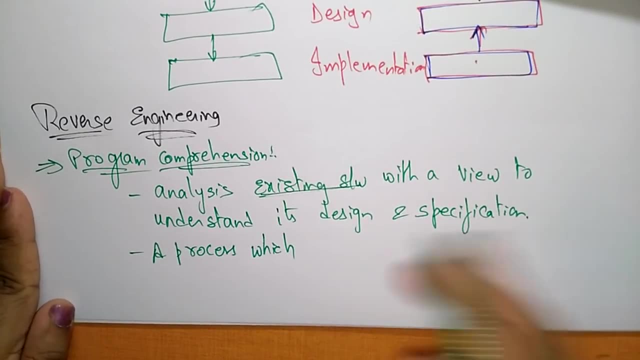 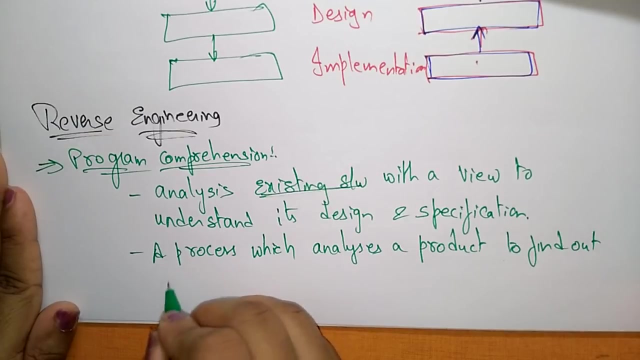 strategy. they can find out how this existing system will be occurred. a process which? a process which analysis a product or a technology. a process which analysis a product or a technology to find out the design aspects and its function. that you is. that is a reverse engineering. you will follow that reverse engineering. 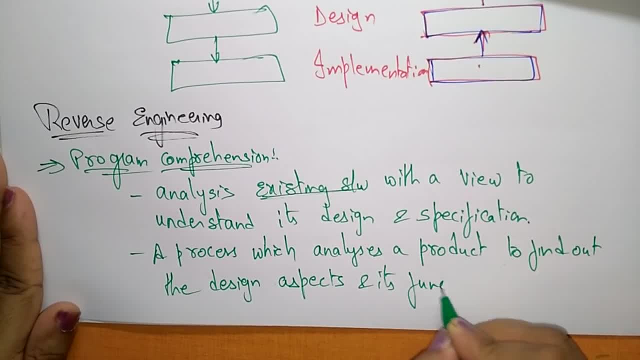 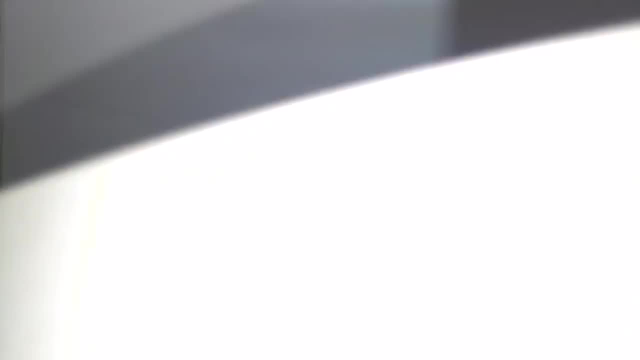 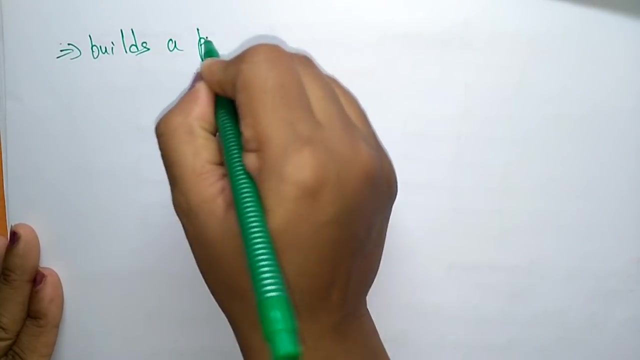 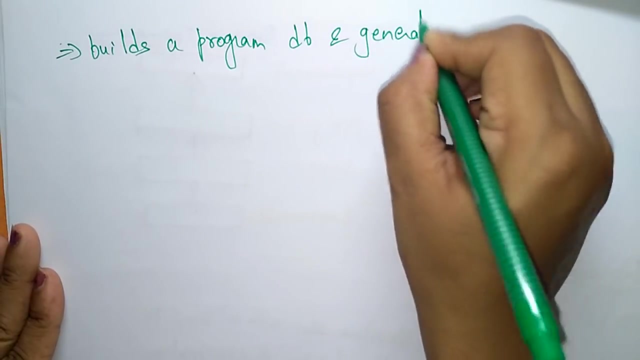 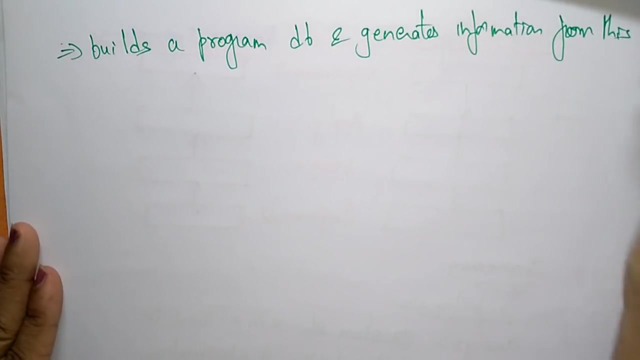 in this case. so whenever you need to find out the design aspects and its functions from this product, you can follow the reverse engineering. it builds a perform. mainly it builds a program database. it builds a program database and generates information from this. so the main useful here is reverse engineering. it builds a program database by taking the 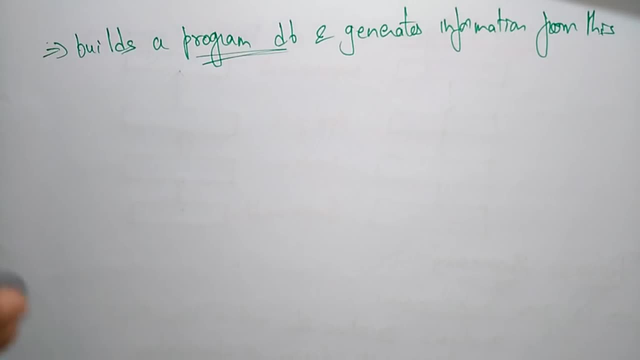 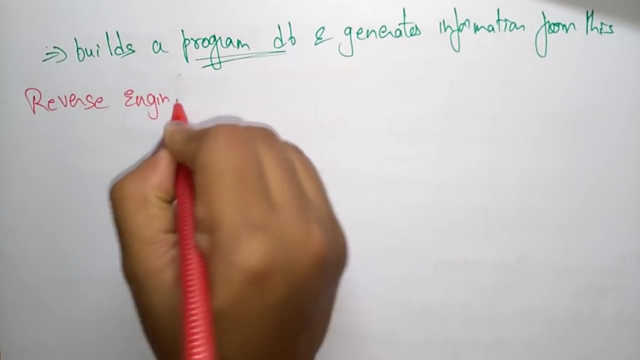 following the reverse strategy, it can able to build the program database and also that program database it's useful for generating the information. now let us see the reverse engineering goals. what are the reverse engineering goals by? by seeing this, I feature so what he here. some people may prefer the reverse engineering strategy. 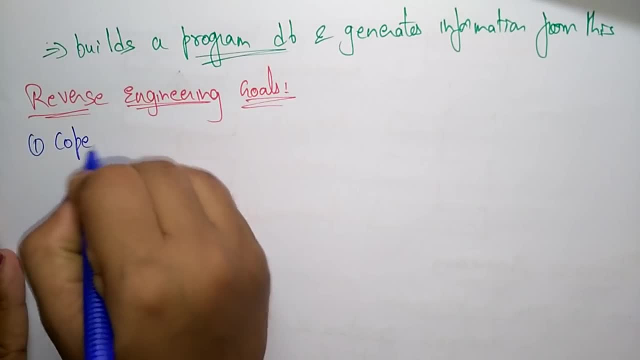 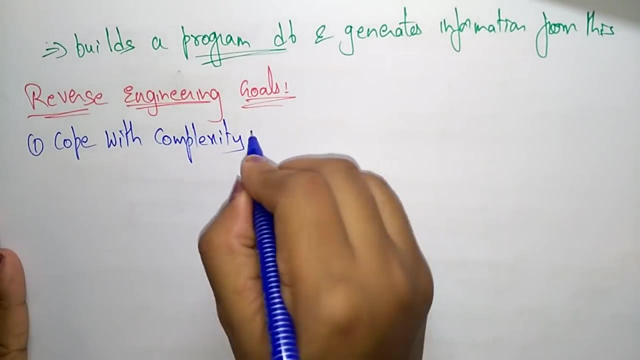 that he was in green goals or complexity. so what it's mean? what it's mean? complexity means sometimes there is needed techniques to understand the larger the complex system. so in those cases, if you go for the reverse engineering, the complexity means there is a cope with complexity. so by adding the new techniques, 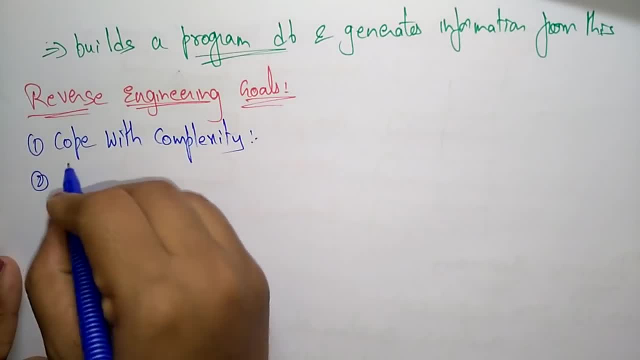 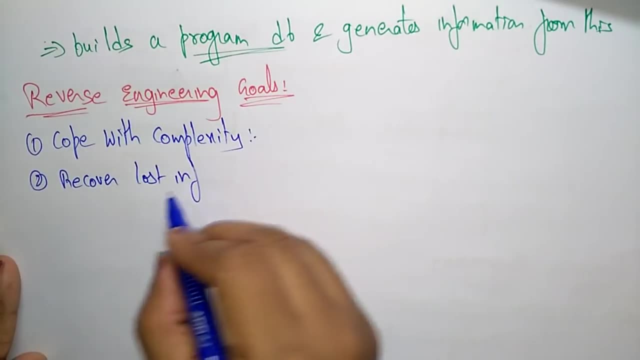 to understand large systems and next recover lost information. recover lost information, so there is a chance of recovering the lost information means extract what changes have been made and why. so with the help of the reverse engineering, you can recover the lost information. okay, suppose if you, if you are going on the road, suddenly you lost your purse. so what you will do? 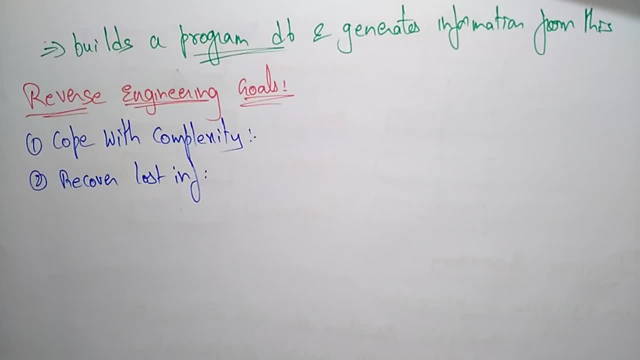 you will just follow the same route back from where you came means you have to reach to that destination. starting point. what you will follow, you just turn out, turn back and start to searching again. that is a reverse back, to recover the lost information, to find out you are valid. 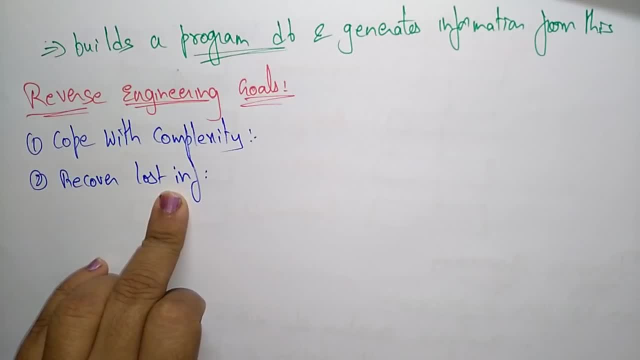 you try to check your the way that you came, okay. so that is the reversing uh engineering goal: to recover the lost information. we will go for the reverse engineering means from coding. they are: check okay, here in this stage. code. what is the problem so here? if it is no problem, okay, it is a problem in the design only. so that's why the code. 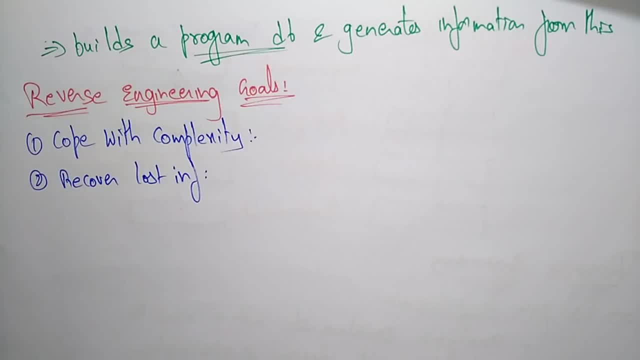 is uh, the it comes a mistake means they check the design. okay, design is also okay. so the problem is only if in the requirements we had we didn't take the exact correct requirements so we have to try to solve the requirements so like that they are going backwards. it's a reverse.